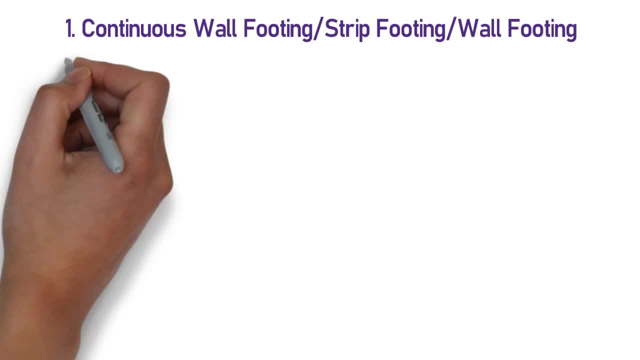 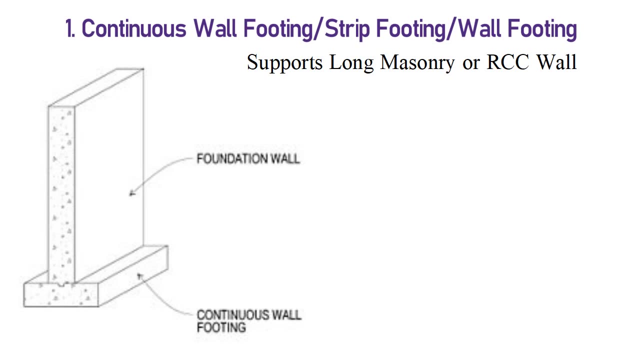 is also known a strip footing or wall footing. The footing which supports a long masonry or RCC wall is known as continuous footing. In this type of footing, the width of footing is twice the width of wall that is rested on it. Sometimes it is even wider. Basically, it runs throughout the length of wall. If 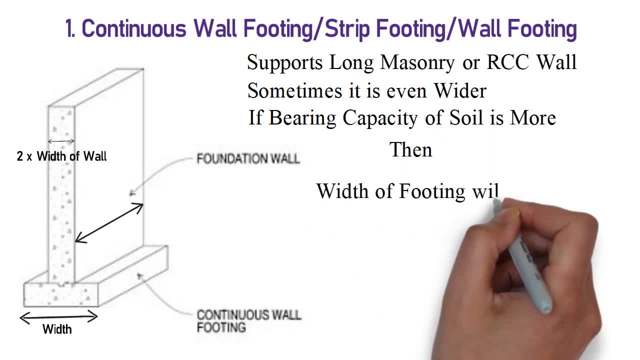 bearing capacity of soil is more, then the minimum capacity of soil is more the minimum capacity of soil is more, then the minimum capacity of soil is more, then width of strip footing will be lesser. This type of footing is generally used in load bearing structures. 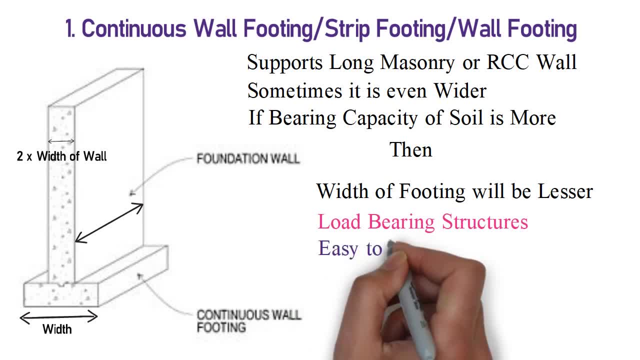 Advantages of this type of footings are: these type of footings are easy to build. It doesn't require skilled labors and expensive tools to construct this type of footing. And if we talk about disadvantages, then the durability of this type of footing is less. 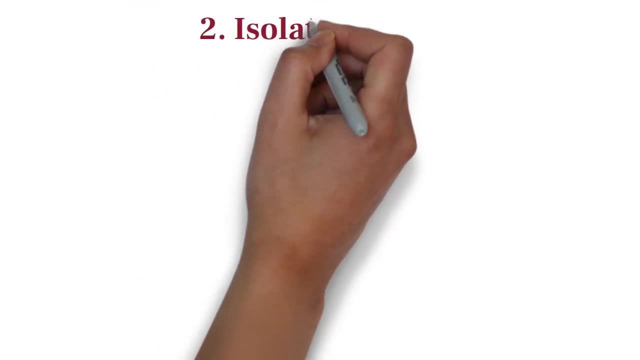 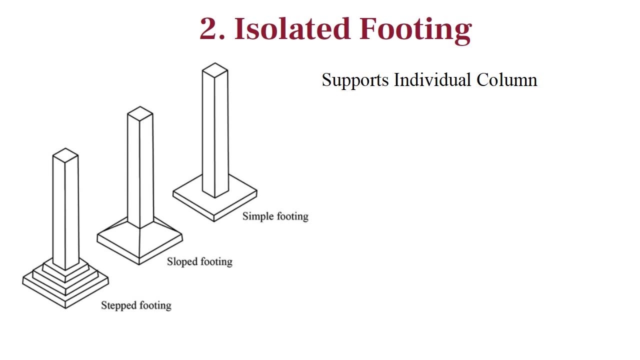 when compared with other types of footings. Number 2,: isolated footing. This type of footing supports individual column. that's why it is called as isolated footing. If good soil is available, then these kinds of footings are economical. The isolated footings essentially consist of a bottom slab. 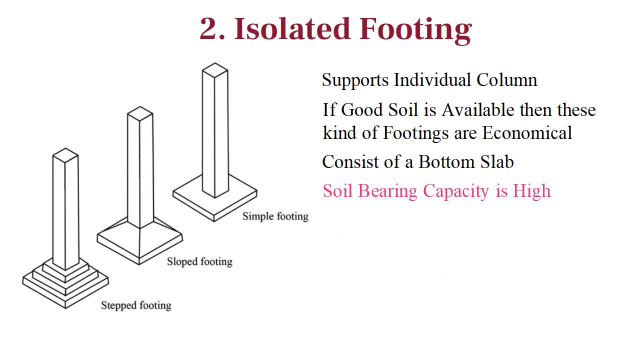 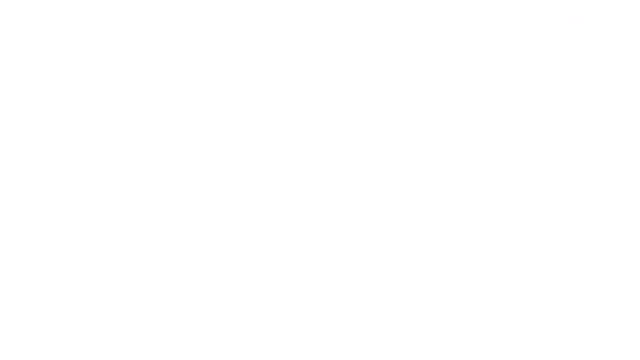 Generally, this type of footings are used when the soil bearing capacity is high, loads on footing are less and columns of a building are not closely spaced. This kind of footings can be of three types, That is simple: Simple footing, sloped footing and stepped footing. 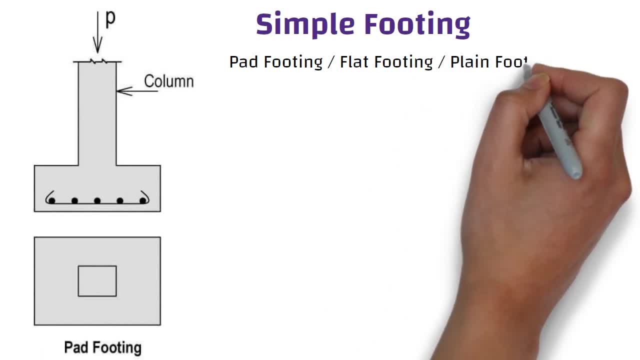 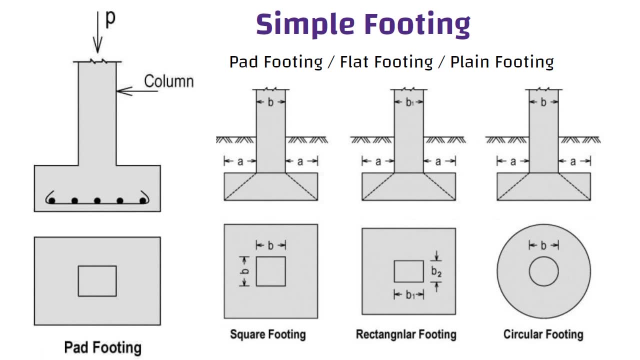 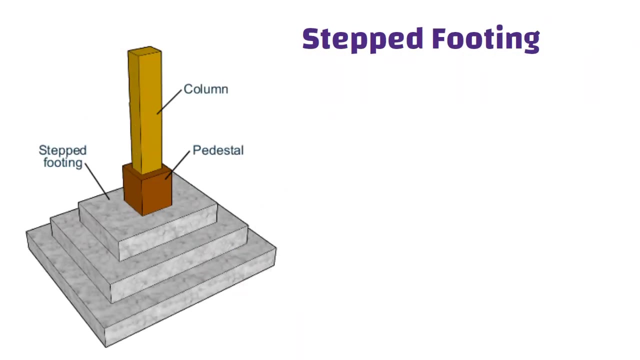 Simple footing is also called as pad footing, flat footing or plain footing. You can see in these pictures this kind of footings can be square, rectangular or circular in shape, which are provided under each column independently Stepped footing. This type of footings were constructed in olden days. now they are outdated. 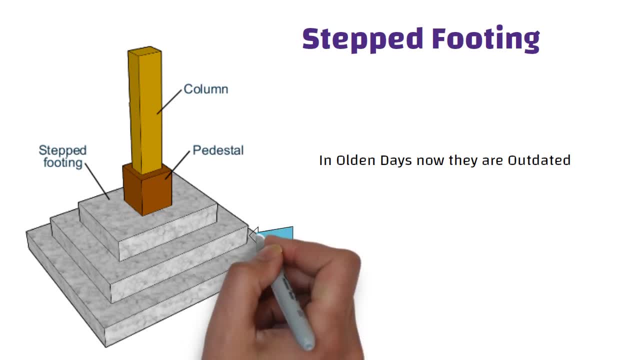 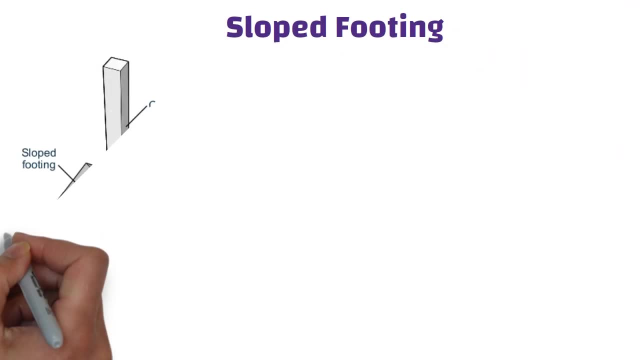 You can see in this picture, three concrete cross sections are stacked upon each other And it forms as steps. That's why it is called as stepped footing, Sloped footing. Sloped footings are also known as trapezoidal footings. 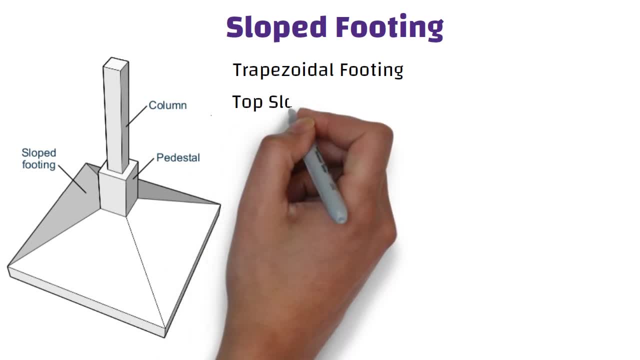 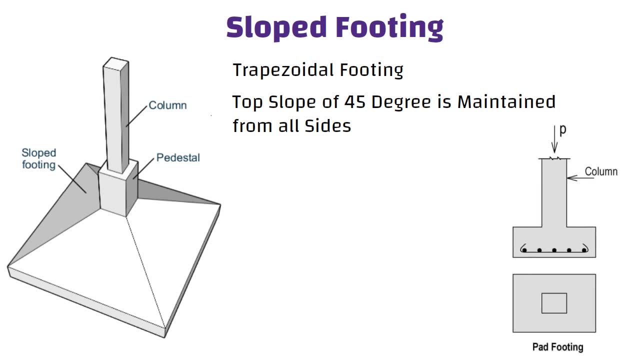 They are designed and constructed with great care to see that the top slope of 45 degree is maintained from all sides. When we compare trapezoidal footing with pad footing, you can see the concrete quantity required to construct. trapezoidal footing is less. 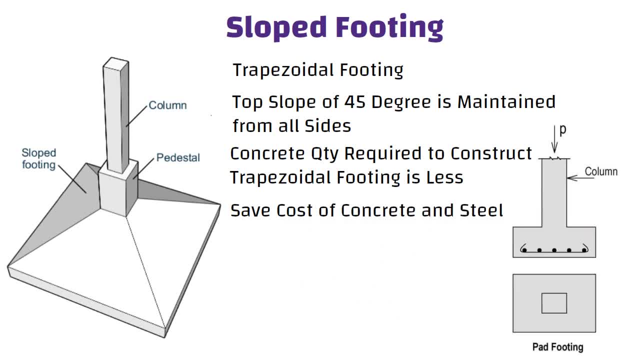 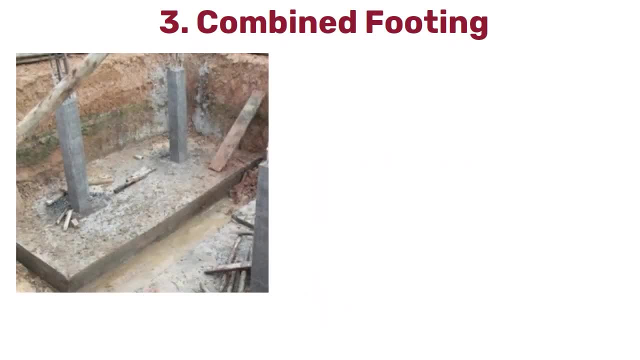 Hence we can save the cost of concrete And steel while constructing this type of footing. Number three: Combined footing. A footing that supports two or more columns is known as combined footing When columns are closely spaced, and in this scenario, if we try to construct individual 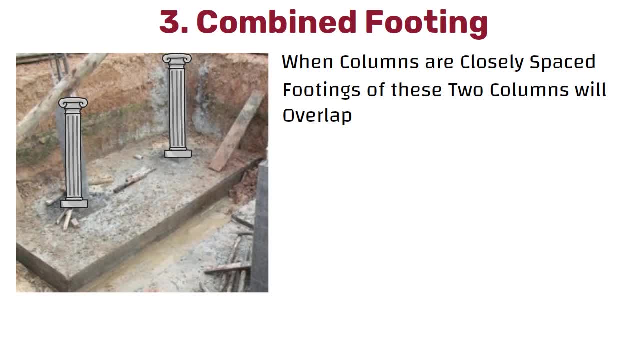 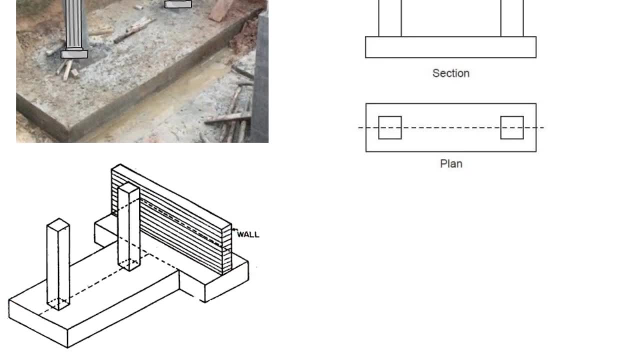 footings, then footings of these two columns will overlap, So in this case it is better to provide combined footing than isolated footing. When one column is close to property line or sewer pipe, The center of gravity of column will not coincide with footing. 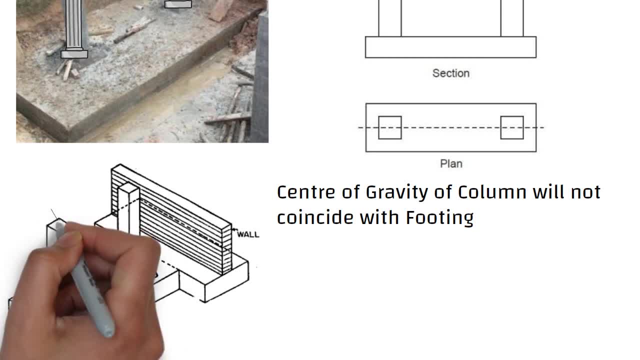 In such cases, it is necessary to provide combined footing with that of the adjacent internal column. The ultimate aim is to get uniform pressure distribution under the entire area of the footings. To achieve this, the center of gravity of footing area should coincide with the center. 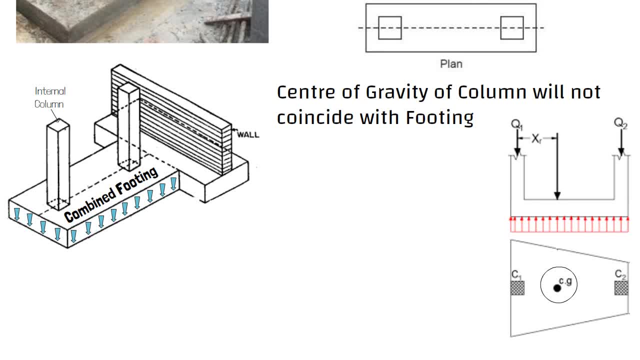 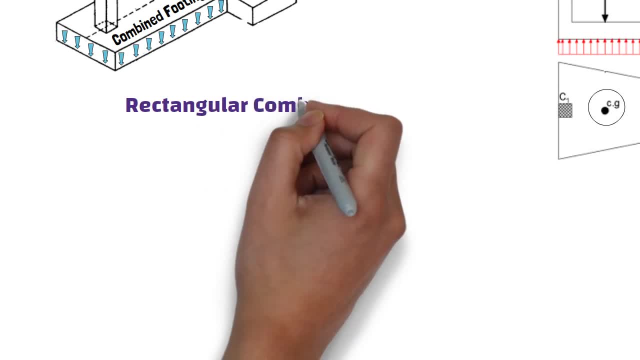 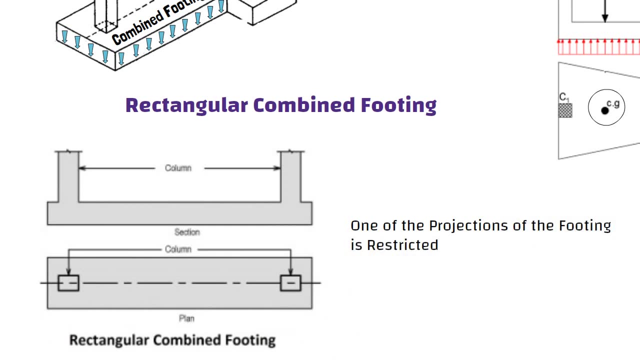 of gravity of total loads of two or more columns. Combined footings are further classified into following types based on their shapes: The rectangular combined footing. The rectangular footing is provided when one of the projections of footing is restricted or the width of footing is restricted. 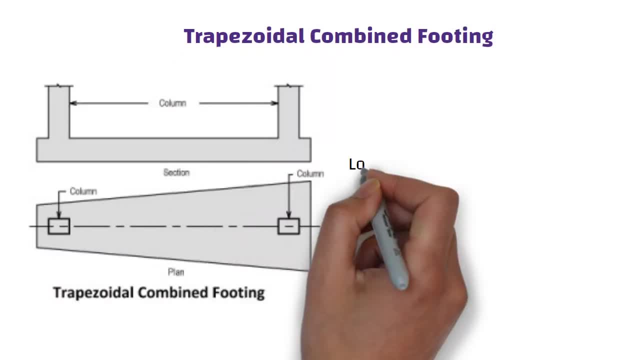 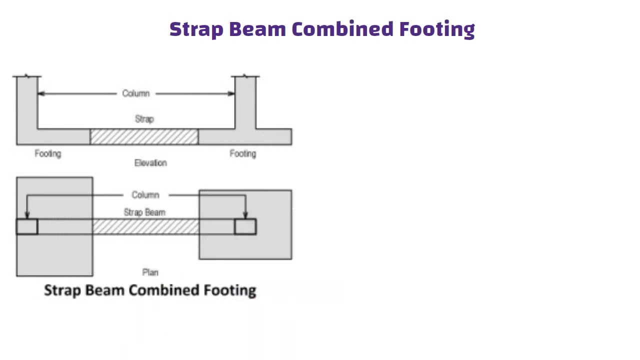 Trapezoidal combined footing. The trapezoidal footing is provided when load of one column is much more than the load of other column. Strap beam combined footing. Strap beam type combined footing is used when one column is located on a property line, resulting. 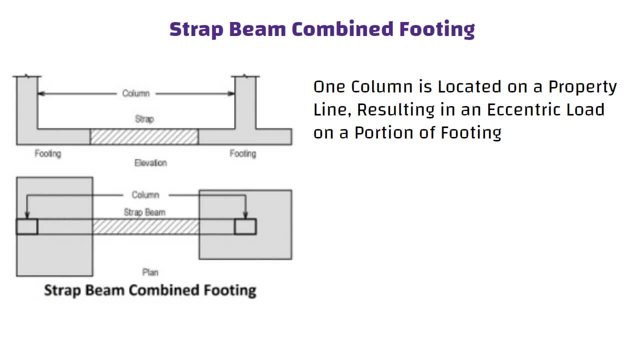 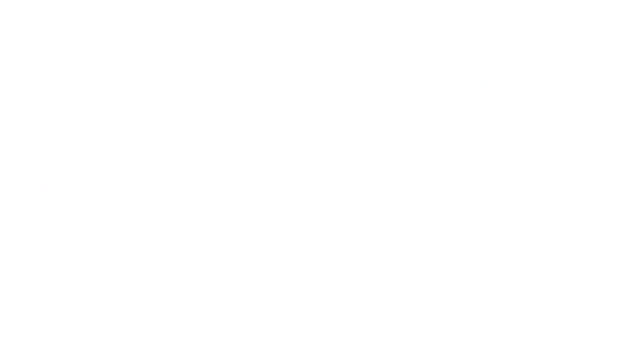 in an eccentric load on a portion of footing. Therefore, in this type of footing a beam is provided to the adjacent column footing to restrain the overturning effect. Number 4.: Raft footing. The raft footing is also called as mat footing. 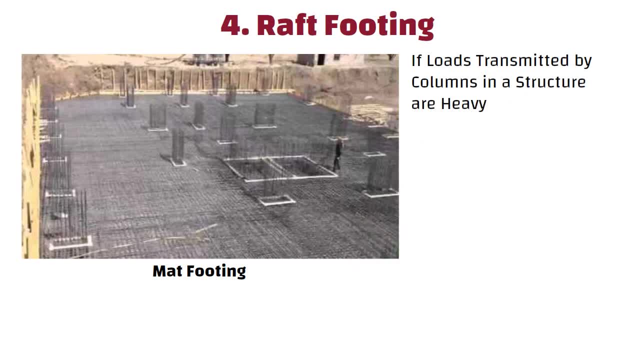 If loads transmitted by the columns in a structure are heavy and the allowable soil pressure is small, then footing requires more area. So, in order to spread the load over large area with less depth, So in order to spread the load over large area with less depth,